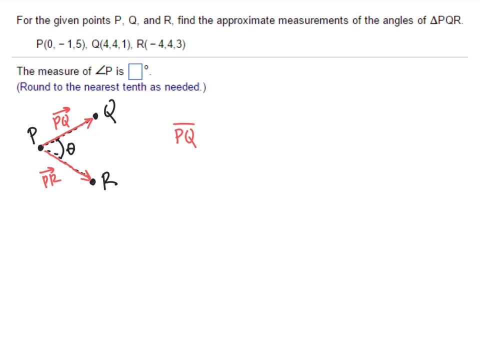 top. So P, Q and R, pq dot, pr is the magnitude of pq times the magnitude of pr, times the cosine of that angle theta that we're looking for. So if we can find those two vectors, pq and pr, then we can take. 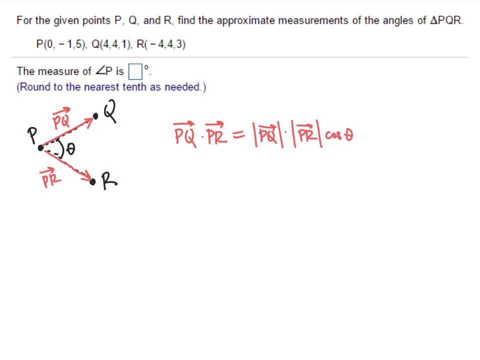 their dot product and then we'll know all of the numbers in this equation, except for the cosine of theta We'll solve. for the cosine of theta, use inverse cosine to get theta itself, and that's our strategy. That's how we're going to do this. So first things first. how do we find pq? 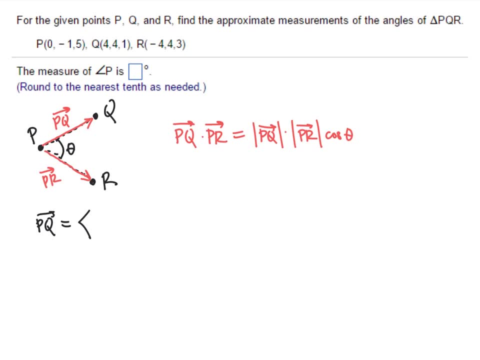 So the vector from p to q is the coordinates of q minus the coordinates of p, So that's going to be 4 minus 0 comma, 4 minus negative, 1 comma 1 minus 5.. So that means our vector is 4, 5,. 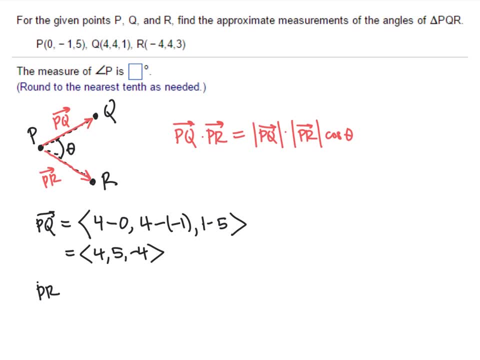 negative 4.. And the vector from p to r is the coordinates of r minus the coordinates of p. That's going to be negative 4 minus 0,, 4 minus negative 1, and 3 minus 5.. That gives us the vector negative 4 comma, 5 comma negative 2.. 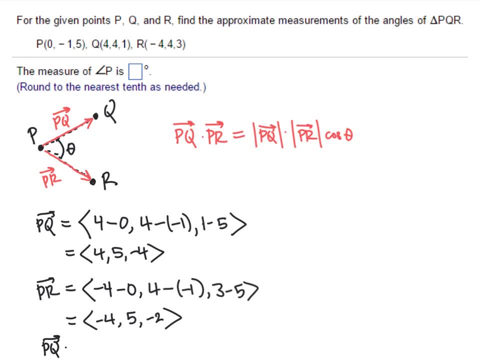 So now we're going to take the dot product, those two vectors, pq, dot, pr, Remember. for the dot product, we're just going to multiply the corresponding components. That's going to be 4 times negative, 4 plus 5 times 5 plus negative 4. 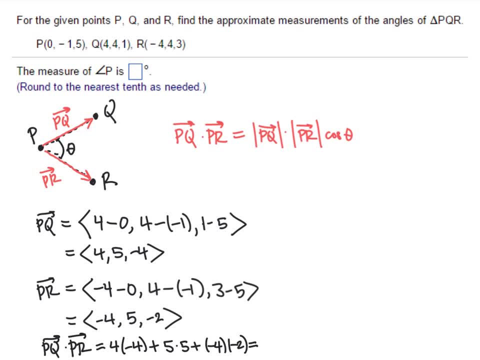 times negative 2, and that's going to be negative 16 plus 25 plus 8, which is 17.. So that's our dot product. So this number right here is 17.. What about the magnitude of these two vectors? So the magnitude of pq is going to be the square. 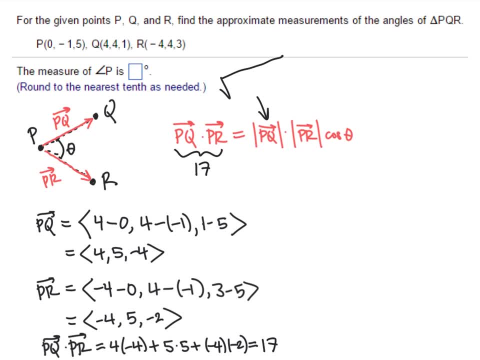 root of the squares of the components of pq. So that's the square root of 4 squared plus 5 squared plus negative 4 squared, which is the square root of 57.. Similarly, the magnitude of pr works out to be the square root of 45..